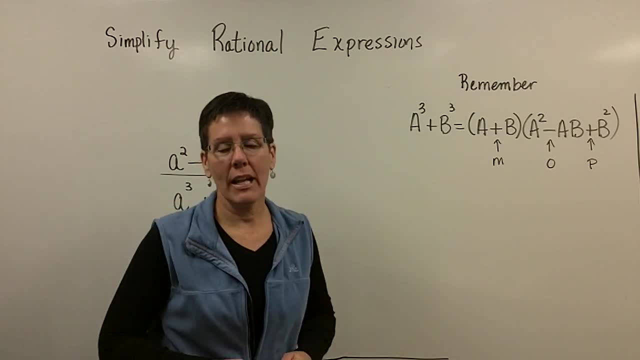 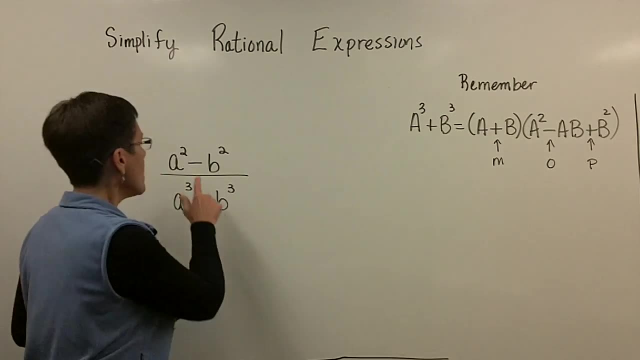 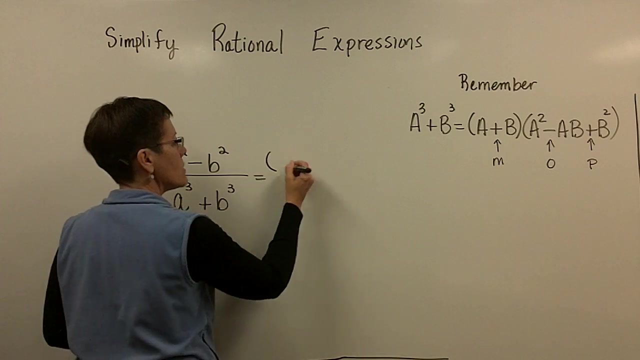 And this sign is always positive. so I use that acronym MOP, to make sure that I factor a cube correctly. The sign matches it's opposite and it's positive. The numerator of this problem is the difference of squares, though, So let's factor that into a plus b, and a minus b Done. 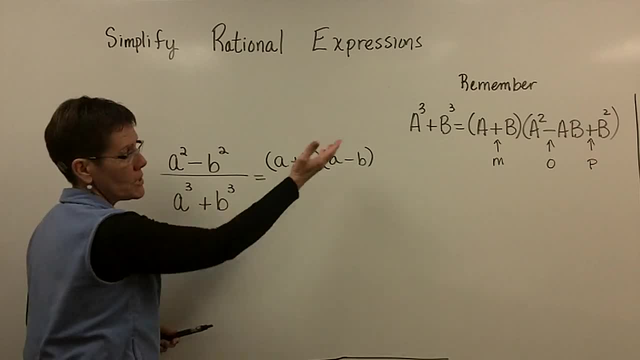 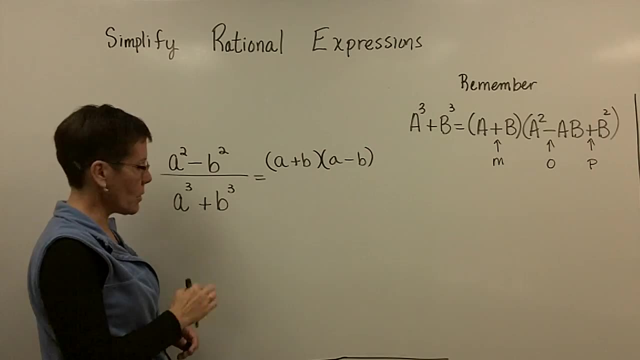 Easy Difference of squares. Here's the sum of cubes and you know, essentially, other than the fact that these are lowercase letters, this is going to factor into that expression. over to the right, The next problem that we're going to do: I'm going to make sure I have some coefficients. 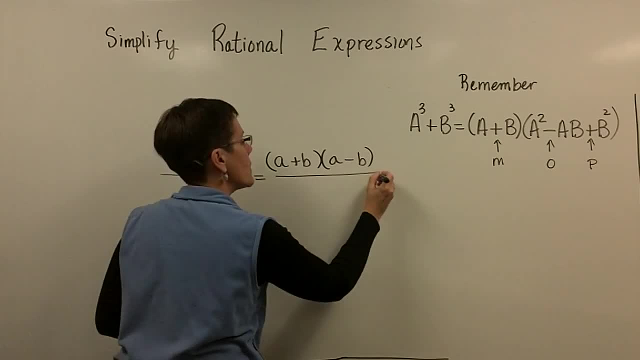 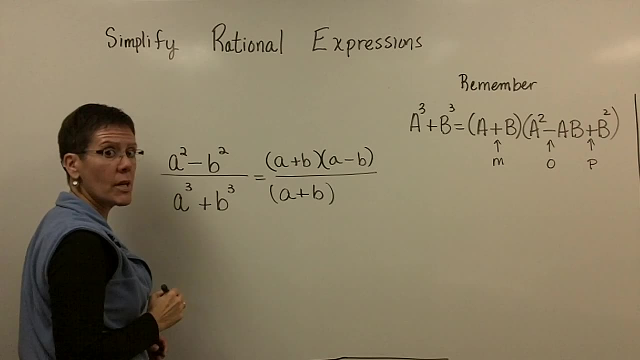 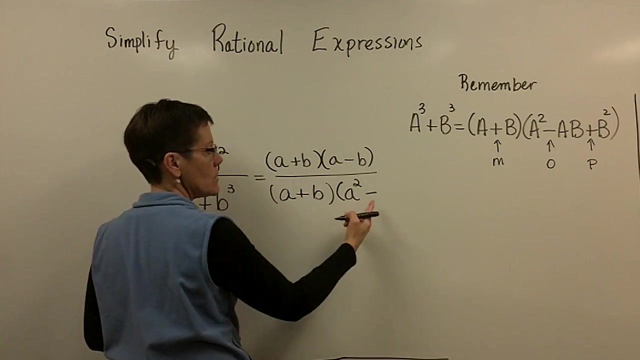 here some numbers in front of the variable. So this expression is going to factor into a little a plus b. Again, over there I have capital A plus b, but these are lowercase variables. And then little a squared minus opposite sign matches opposite and then positive. So I've got the 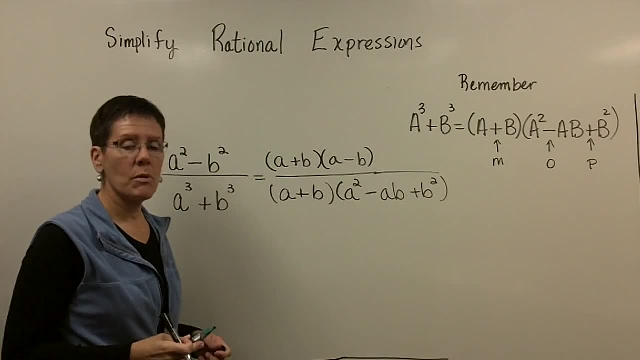 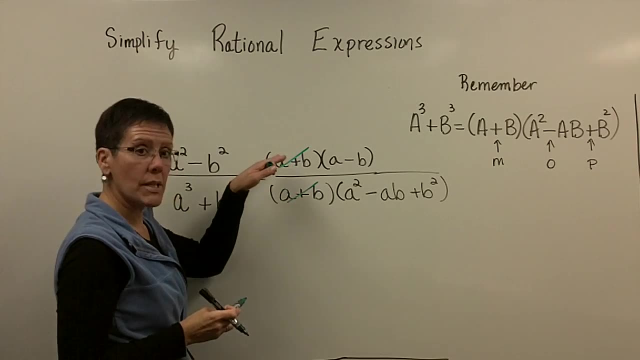 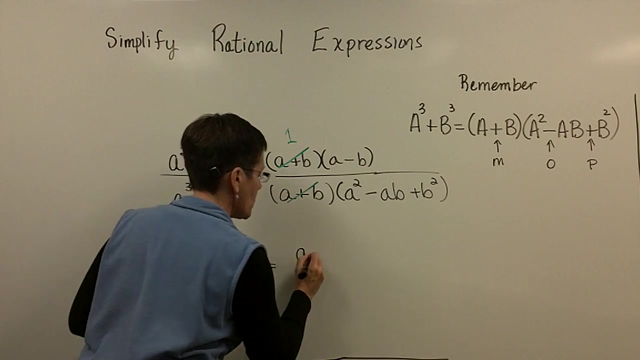 numerator and the denominator factored, And once I've done that, remember that you take out a common factor. It is equivalent to: it is like saying I'm removing the number one because that's a plus b over a plus b, So I'm taking out a one. So all I have left in this numerator is the a minus b and then the a. 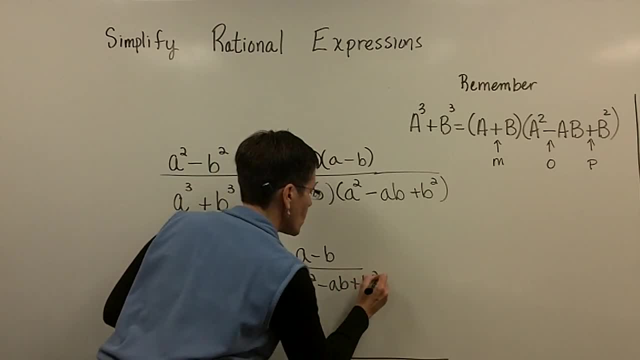 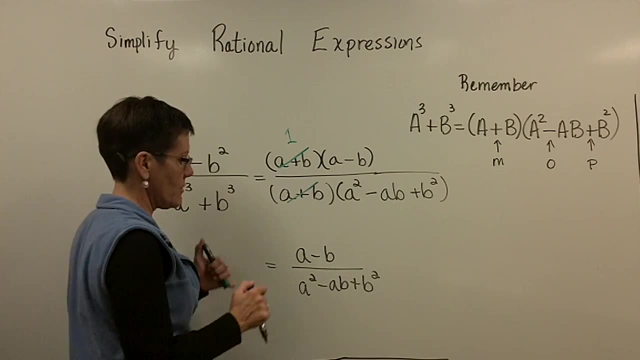 squared minus the ab, plus the b squared. This is not factorable again And if you didn't know why, you could use the AC method to determine that. There's no way to find two numbers whose product is one that adds to be a minus one. 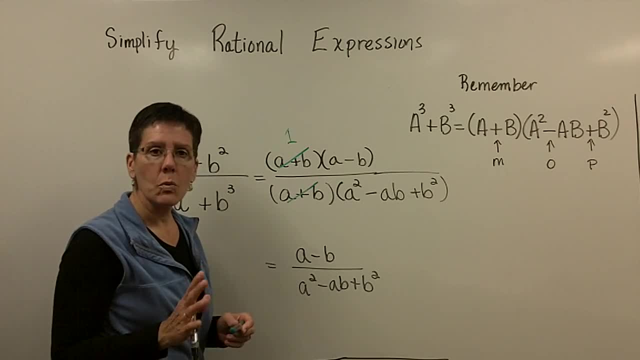 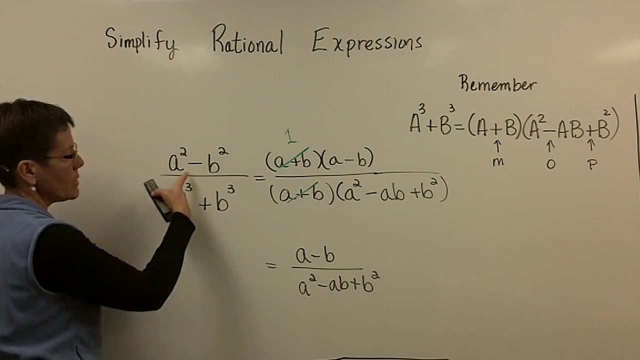 Because product is one, has to be one and one. Those will always add to be either two or negative two. so they can't add to be that one. right there, Let's do another problem. So here we have the difference of squares and the sum of. 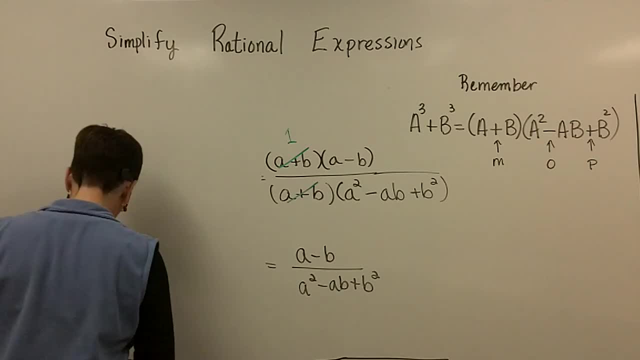 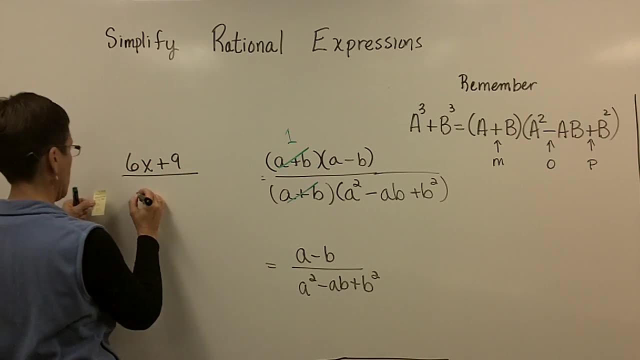 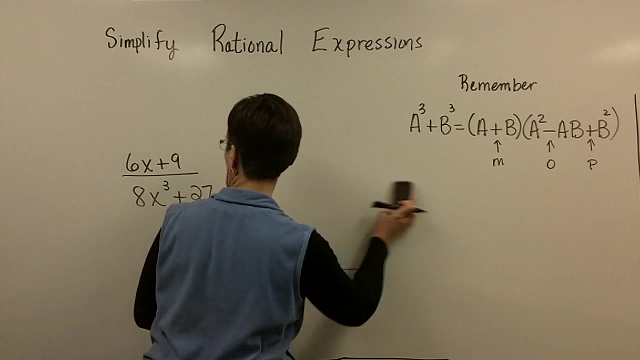 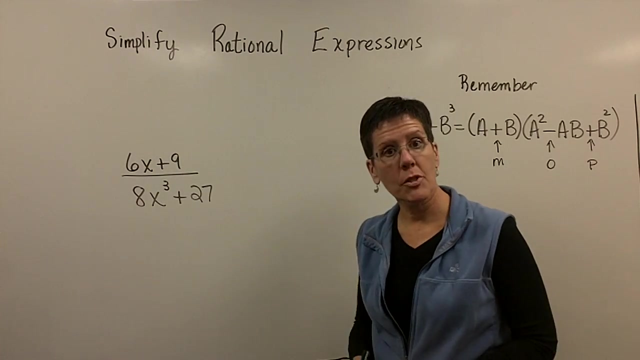 cubes. I'm going to go ahead and put the problem up while you're maybe finishing, So let's go. And it happens that in this problem I happen to have a sum of cubes again. I probably should've made that a difference of cubes and I wasn't thinking there. But 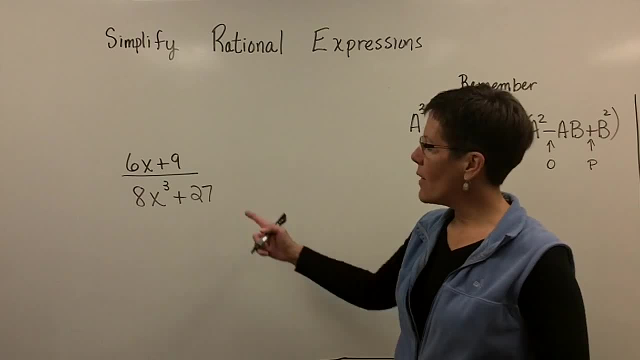 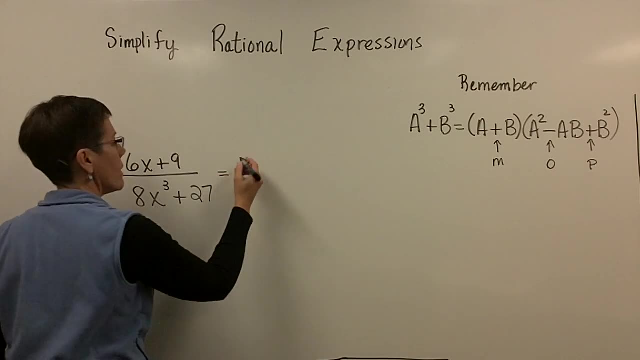 let's go ahead and factor the numerator and factor the denominator. The numerator in this problem just has the greatest common factor in it of a three. So alright, let's get the, the 3 out of there, So we'll have 3 times the 2x plus 3.. And then down here I have 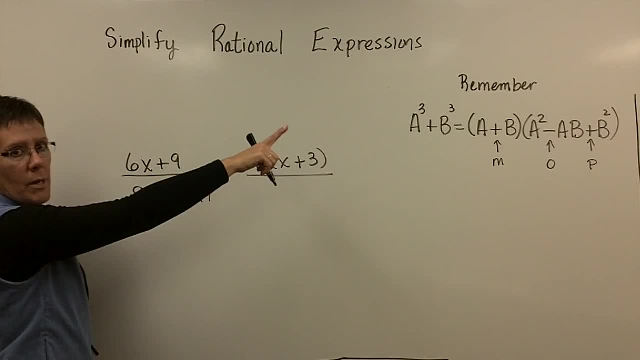 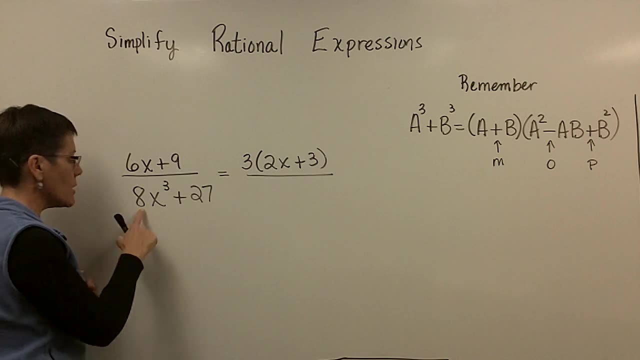 to determine what my A value over there and my B values, my capital A and my capital B values, are. This is real hard for some folks and I'm just going to help you practice with that factoring thing again. One thing you could do is you could get your calculator. 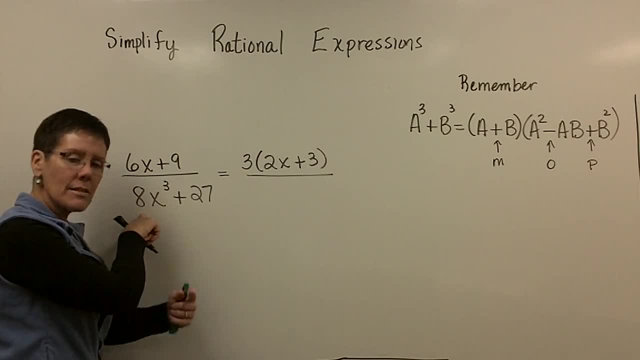 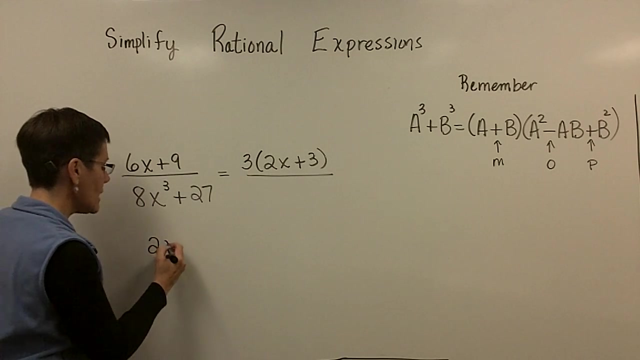 out and find out what the cube root of 8 is. I'm asking you, though, what is the cube root of 8?? I'm asking you, for what number times itself 3 times gives you 8? And 2 is that number 2 times itself 3 times gives you 8.. And then you know what letter times. 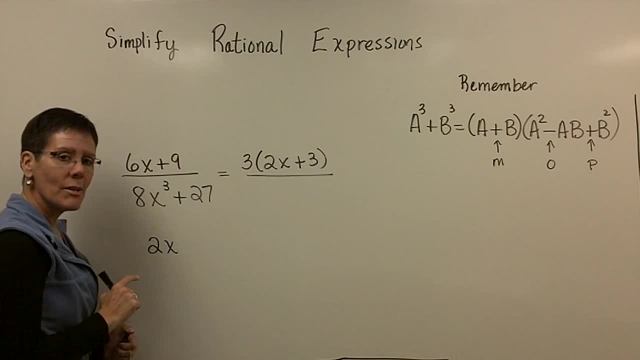 itself 3 times gives you x to the 3rd And that letter is x. So the factor 2x if you cubed it, this A value if you cubed 2x, 2x times 2x. 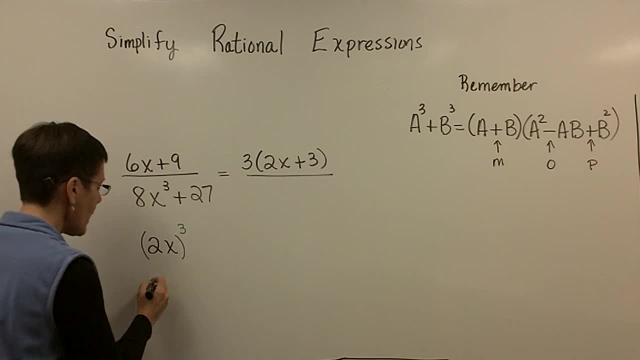 2x times 2x is 8x cubed. So my A value that I'm going to put into this problem everywhere is going to be the expression 2x And the cube root of 27 is the number 3.. So in other, 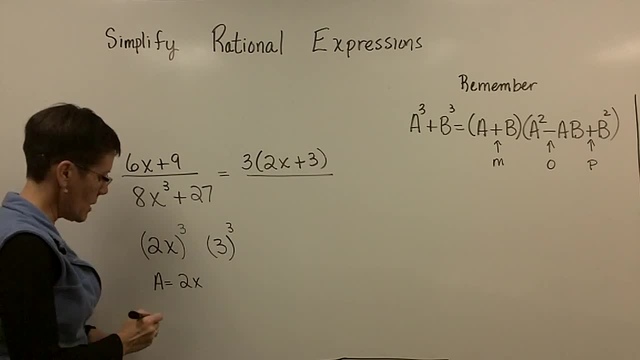 words 3 cubed gives you 27.. So my B value for that formula over there has to be the number 3.. So that's how you find your A and your B value. Now you just stick the 2x and the 3 in here. 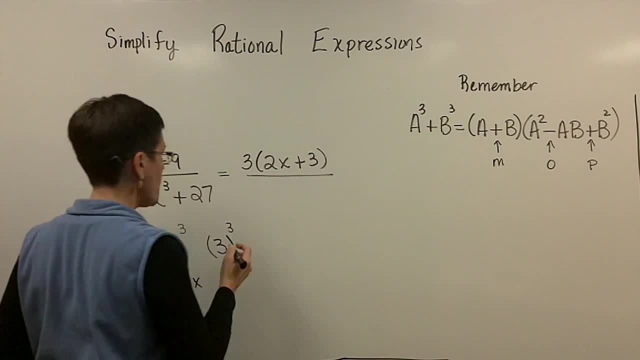 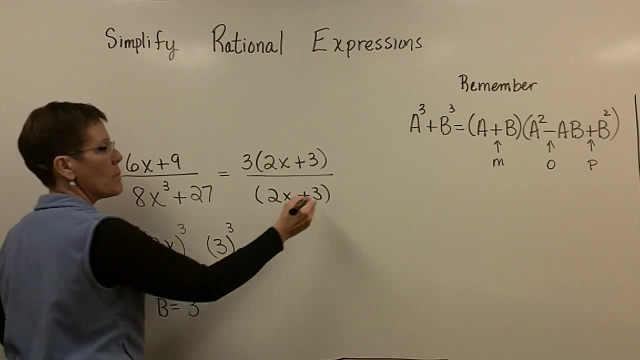 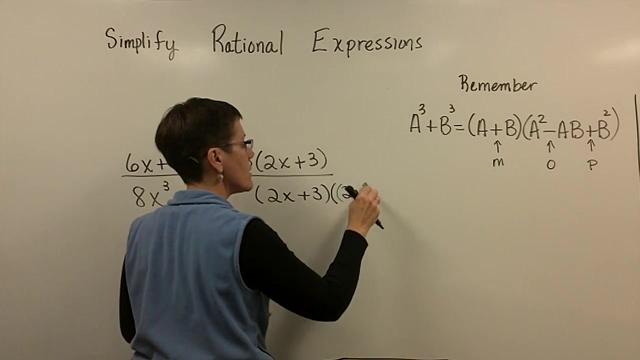 Anywhere you see A and B. So it's pretty easy for the binomial. The binomial is going to be the A value plus the B value, That's 2x plus 3.. But be careful here. You have to take the 2x, which is your A value, and you have to square it. So that's going to be 4x. 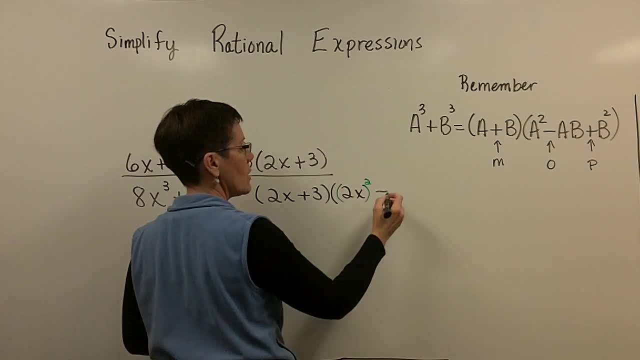 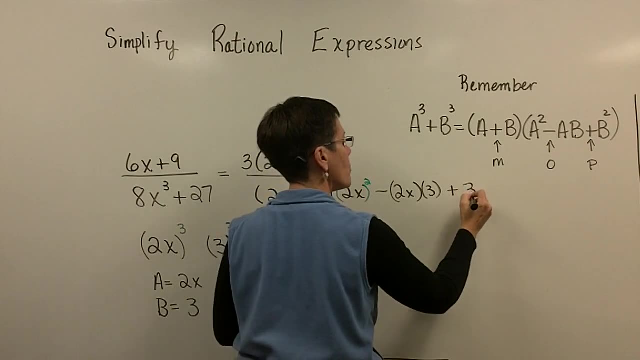 squared. And then we have to have an opposite sign here And we have to take our A value times our B value, which is 3.. And then finally, always a plus sign right here, And then we have to take our B value squared, which is going to be 9.. I'm going to go ahead and write.